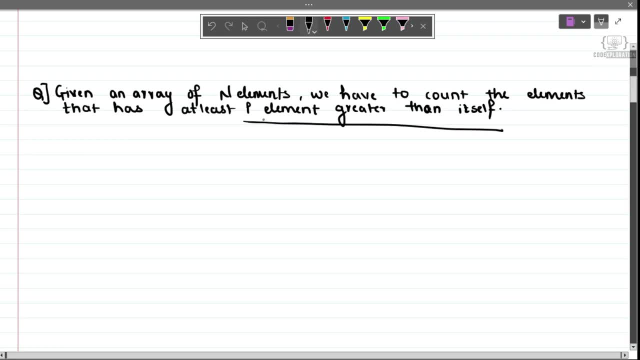 Now let me explain you this question with the example. Let's say we have an array that has the element as one, six, three, nine, five, eight, two, ten and four. Let me give you the indices: zero, one, two, three, four, five, six, seven, eight. Now. 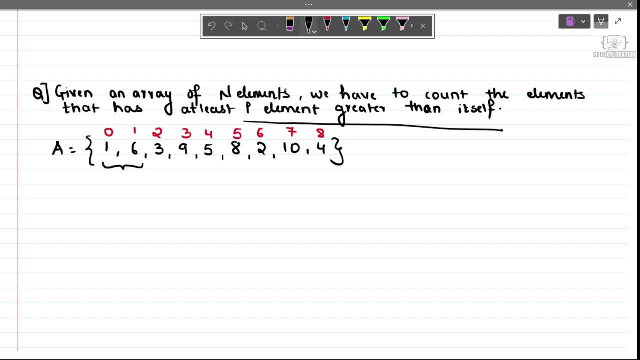 if we see the first two elements now, six is greater than one, so here six is greater than one, so one will be the output. Why one? Because in these three elements one element is smaller. Now, if we take first 3 element, then 6 is the largest element here and 1 and 3 are smallest. 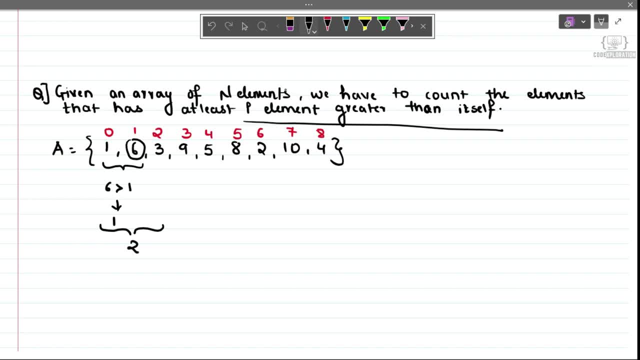 so answer will be 2.. Now, if we take the first 4 element, then here 9 is the largest element and 1,, 6,, 3 are the smallest element. Similarly, if we take first 5 element, then here also element 9 is greater than 1, 6,. 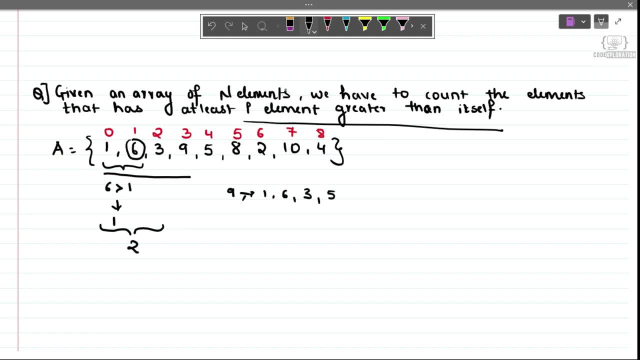 3 and 5, so answer will be 4.. Now, if we consider the whole array, here, the largest element is 10 and the length of the array is 10.. So if we subtract 1 from 9, then the answer will be 8.. 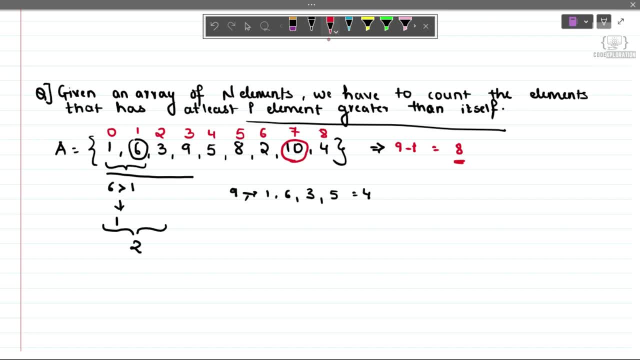 So there are 8 elements which are smaller than 10.. Now let me take some another example here. the element will be minus 7,, 2, 10,, 3,, 4, 10, minus 5, 10,, again 3, minus 3, 9, minus 8 and minus 1.. 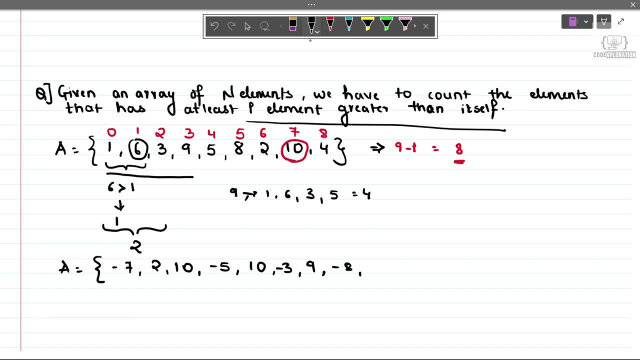 So pause the video and see what will be the answer. So here the maximum element is 10 and we have 2 tenths here. Let us now see the answer. So here the maximum element is 10.. So here the maximum element is 10.. 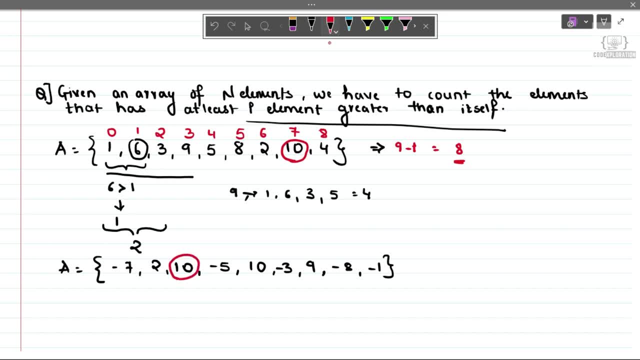 And we have 2 tenths here. So here we have 2 tenths and 10.. So here we have 2 tenths and here the length of the array is 9 also. so there are almost 7 elements which are less. 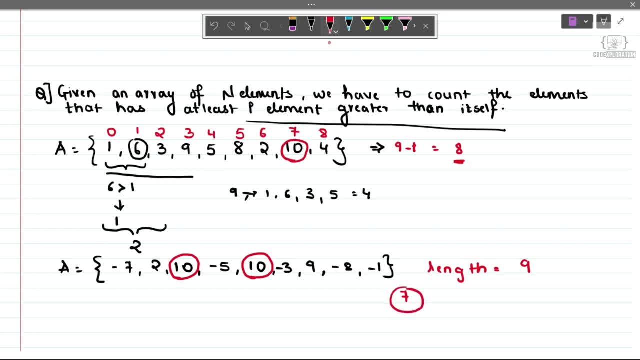 than 10. how 7? now? the length of the array is 9, and if we subtract 9 minus 2, then we will get 7. so this too is the count of the maximum element, that is, 2 times 7 present here. now let me give another example. 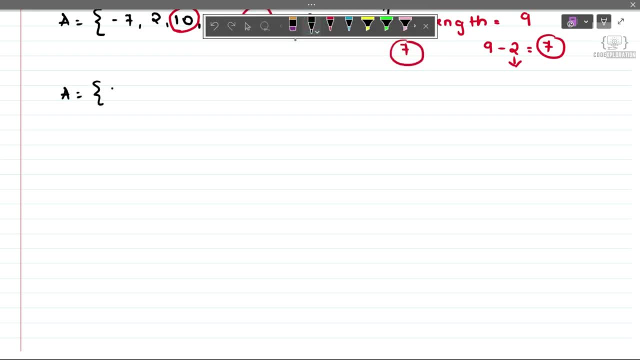 a s, four, four, four, four and four. now again, pause the video and try to solve the problem. so here the maximum element is four and none of the elements are lesser than four, so answer will be zero. now, if you observe, solution will be: get the maximum element from the array. 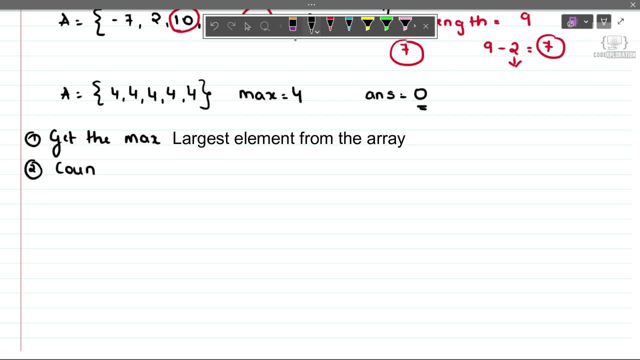 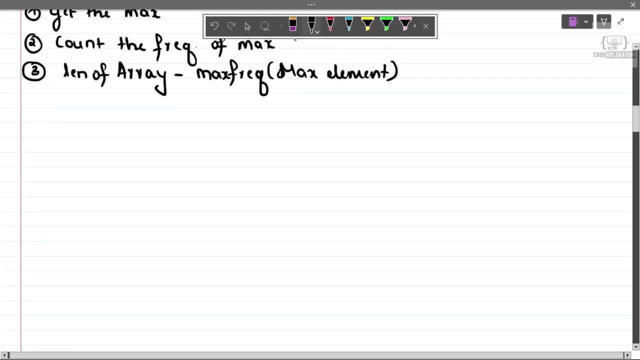 then count the frequency of the maximum element and subtract count of the maximum element from the length of the array, and then the variable will solve it. so the algorithm will be: for i equals to 1, i is less than i plus plus. now here we will initialize the max. 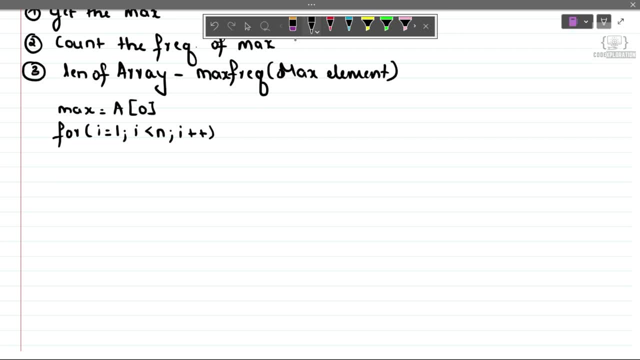 element as the array of zero. now, yes, we did that. now, if you know something about the program programming, you will know how to know. in this video, we will ل الي not just giving you the much of the algorithm, but making the出來 only of object always opposed to the other one is called the desired foreign one. now, if you know something about the program programming, you will know how to find the work within the program. 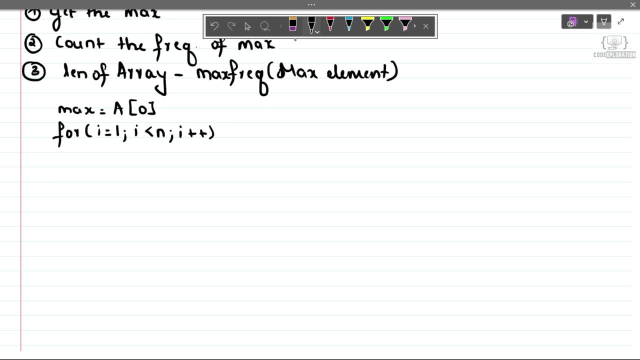 you will know how to find the maximum element from an array. if max is less than a, then we will update the maximum element. from here we are getting the maximum maximum element. now we have to count the frequency of the maximum element. again, we will use the for loop. 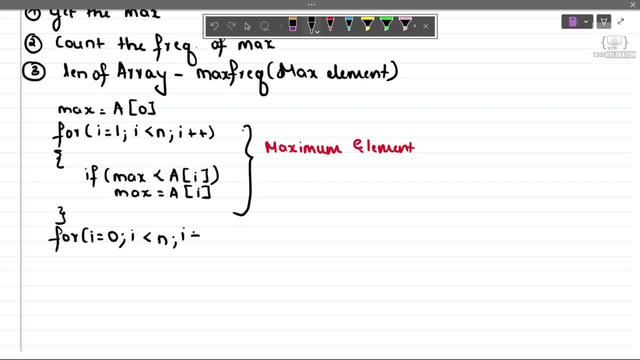 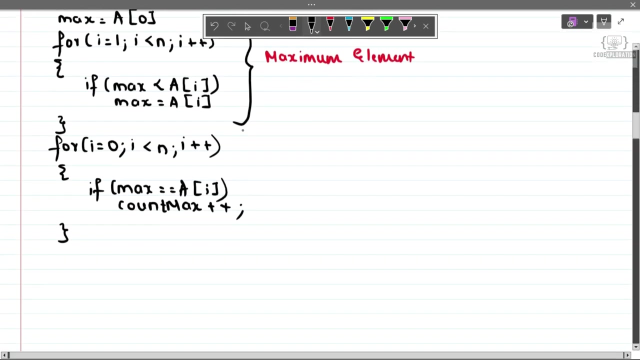 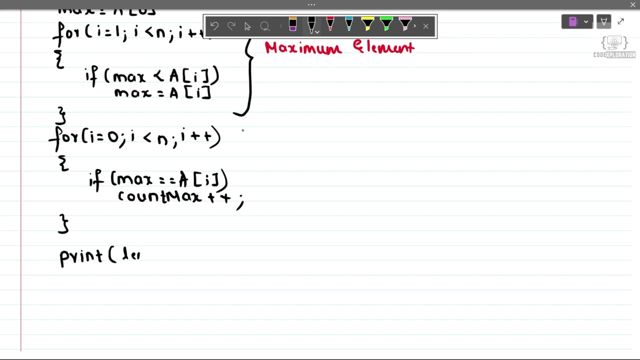 i is less than n, i plus plus. now. here n is nothing but the length of the array. if max equals to a of i, then we will count, increment the maximum. now we will return or print length minus count of maximum element. so this will be the answer. here is the to-do task for you. 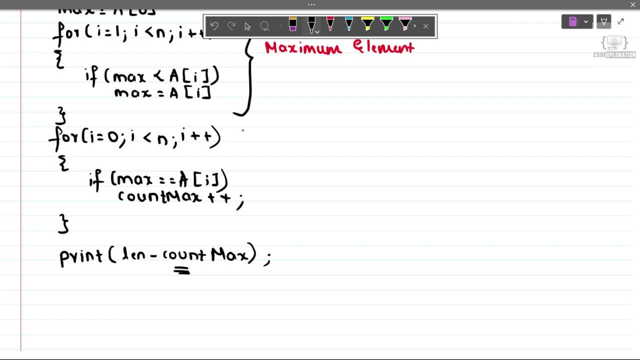 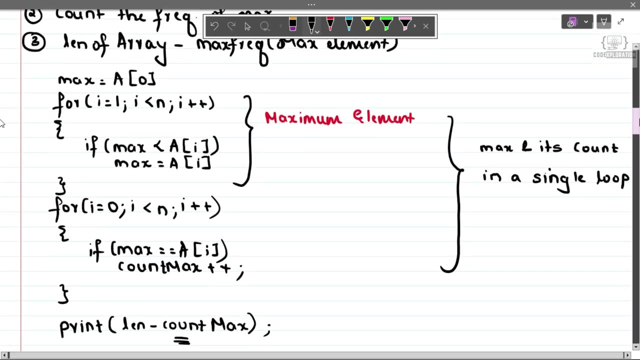 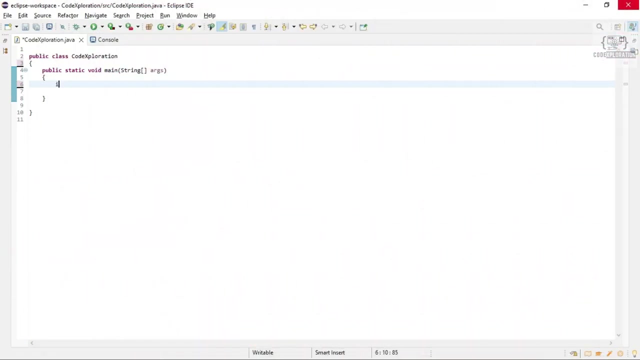 try to come up with the approach that we get a maximum element and its count in a single for loop. so now let's jump to the programming part. now let's initialize the array in a of i. elements of array will be minus seven, two ten minus five. 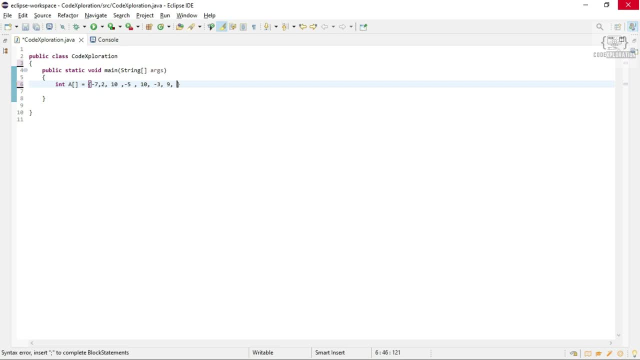 ten minus nine minus eight and minus one. now we have seen this example. so the answer will be count, length of the array minus the frequency of the maximum element. that will be. length of the array here is nine and the count of the maximum element is two. so nine minus two will be seven. now 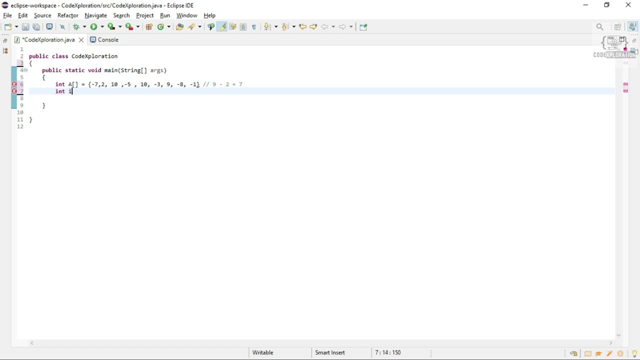 let's initialize some variables. i for the for loop length that will take the length of the array max. that will hold the maximum element. initially the maximum element will be a of zero and the last that is count of max. that is frequency of the maximum element that will be initially. 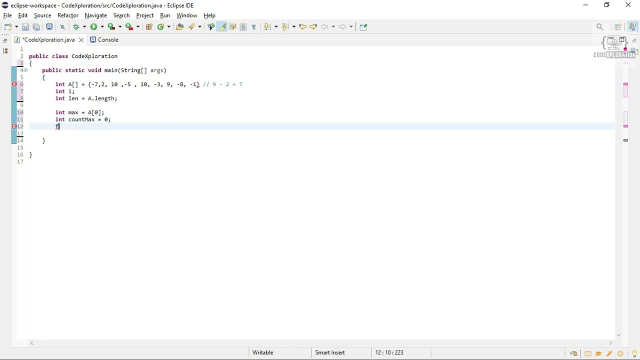 zero. now we will find the maximum element. if max is less than a of i, then we will update the max element. now, here we will count the frequency of the maximum element. what I close to 0, I is less than then I plus plus. if a of I equals to max, 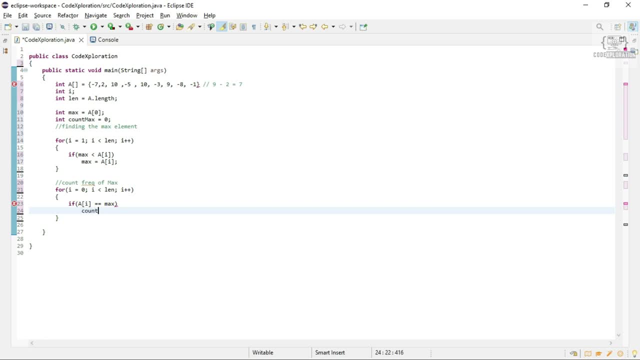 maximum element. if max is less than a of i, then we will update the max element, then we will increment the countmax. now, finally, we will print the answer: length minus countmax. now let's run the code. here is the error. yes, the answer is 7. now the time complexity.